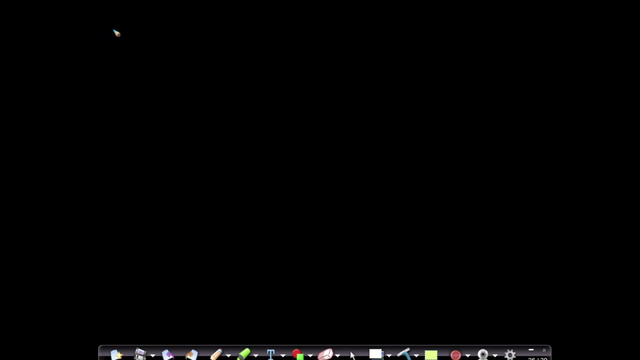 Since we just learned about a point or a vector, let us go slightly ahead and understand the next big idea called a line. It may not sound very big, but let us see how the idea transpires when we look at 2D, 3D and higher dimensional spaces. So let us look at what a 2D line is. Suppose if 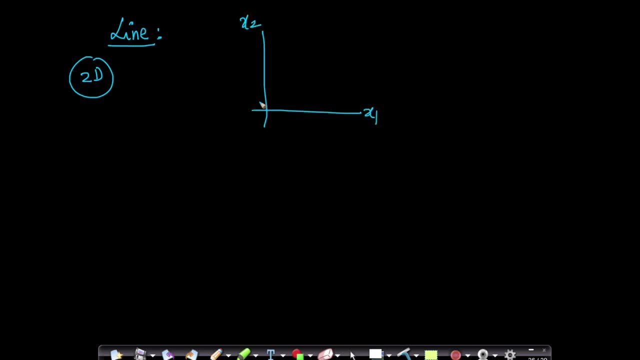 this is your x1 axis and this is your x2 axis. let us say a line here. If you remember your 10th grade math or 11th grade math, we always wrote our line as y equals to mx plus c. If this was x, if my x1 is x, if my x2 is y, I could write my y equals to mx plus c, where m is. 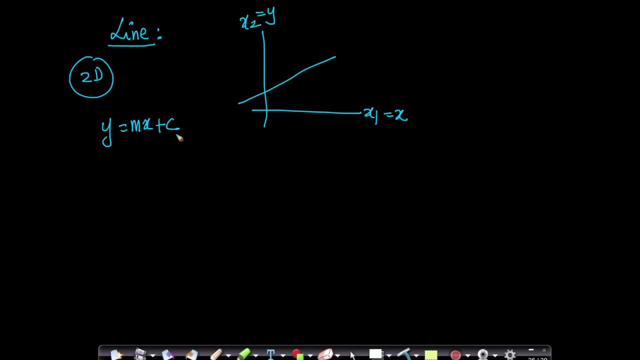 the slope and c is the intercept on y axis. This is one equation of line that we all recall and remember. There is an other equation of line called ax plus by plus c equals to 0. This is called the general form of an equation of a line. 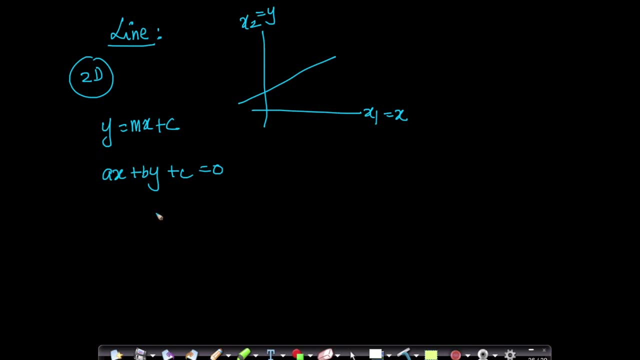 And they both are equivalent. You can prove it because by just rewriting this equation slightly. I can write it as: y equals to minus c by b, minus a by b x. In such a case what happens is this becomes your c here and your m is nothing but this term here. So this is called the general. 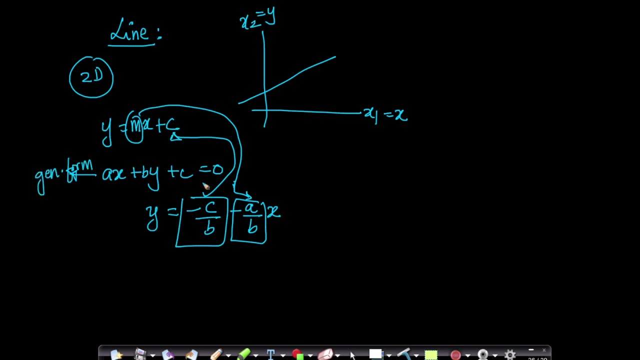 form of general equation or the general form of a line. We will stick to this. We will stick to this notation because it is easier to interpret and this is much more general. If my axes are x1 and x2,, I can rewrite this equation as a times x1. 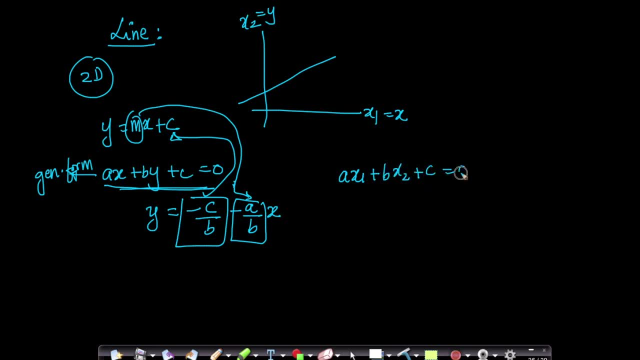 plus b times x2 plus c equals to 0.. Instead of using a, b, c, let me use a different notation, because if you want to do it in 10 dimensions, how would you write it? I will have to use all. 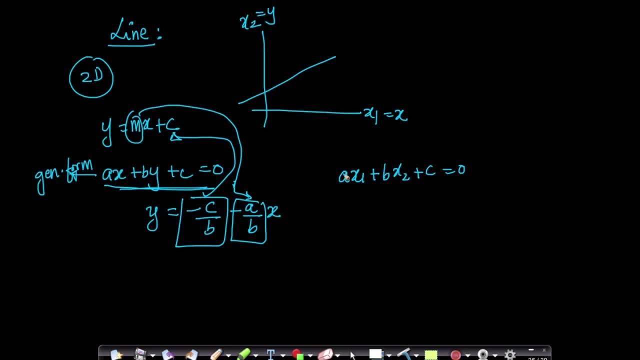 the alphabet. If you want to use 100 dimensions, I do not have enough alphabets, So I will write it as I can write. as w, W1, x1 plus w2, x2 plus w0 equals to 0. So I made: instead of a, I am writing w1.. Instead of b: 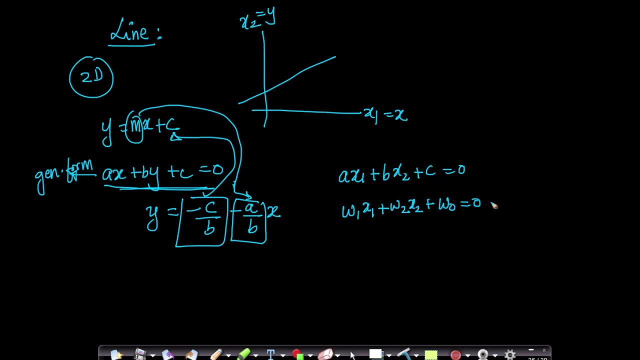 I am writing w2.. Instead of c, I am writing w0.. This is the equation of a line in 2D. What about 3D? Some of you might have learned 3D- coordinate geometry- in undergrad first year math course or probably in some cases even undergrad second year math courses. For those, 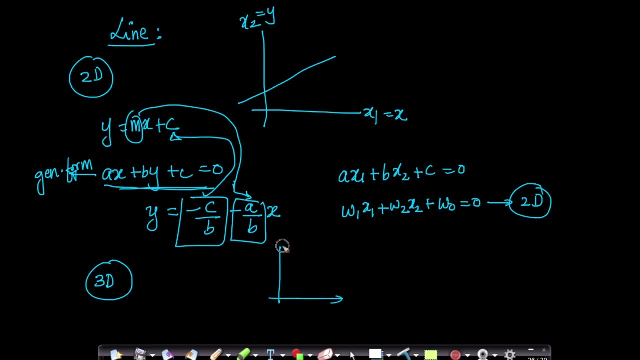 who do not know if I have 3 axes, if I have my axes as x1, x2 and x3, the equivalent of a line. so line is a linear surface in 2D. The equivalent idea of a line in 3D is a plane. 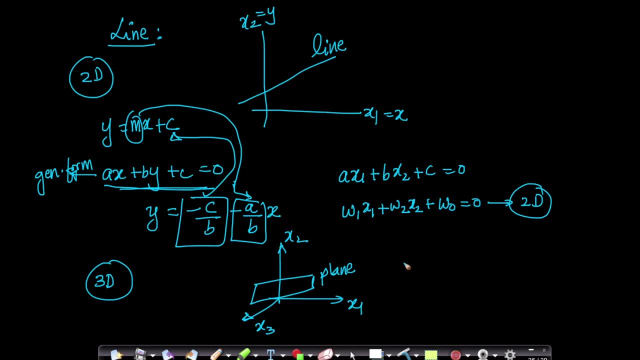 And the equation of a plane. for those of you who might remember it, looks like this: ax plus by plus cz plus d equals to 0. This is an equation that some of you may be familiar with because you took a math course in your undergrad first year and second year. Let us just generalize it. What this looks like is: 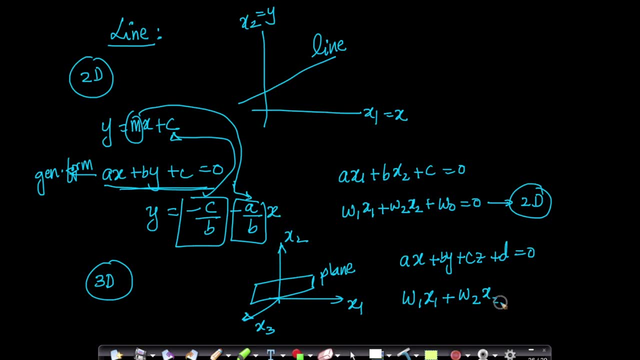 w1, x1 plus w2, x2 plus w3, x3 plus w0 equals to 0.. This is the equation of a linear surface. This is the equation of a plane. This is a plane, This is a line, The idea, the equivalent idea of a. 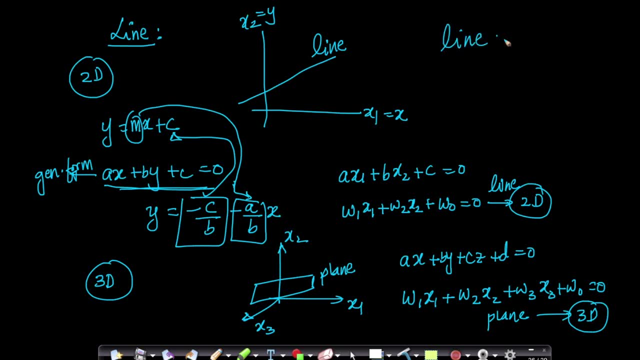 line in 2D is plane, So line in 2D is nothing but plane in 3D. Now the immediate question is: what about n-dimensional space? What is it called? It is called something called a hyperplane. 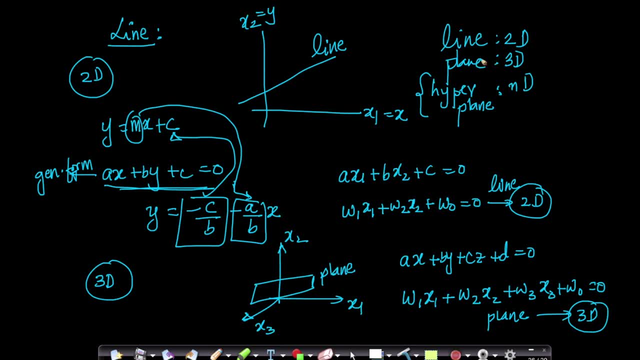 Hyperplane is basically a generalization of the concept of a line or a plane to higher dimensional space. Because, if you think, line is called a linear surface because it separates your plane with a simple linear structure, like a line or a plane, into two regions: one region on one side. 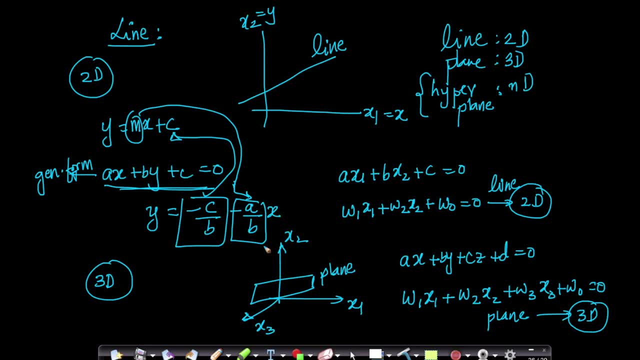 of the line, the other region on the other side of the line. Similarly, plane can separate your 3D volume into two regions, one above the plane and one below the plane. So the immediate question is: what is the equation of a plane in n dimensions? Suppose if I have n dimensions. 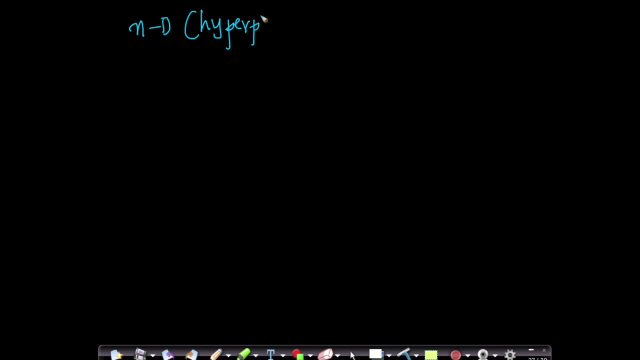 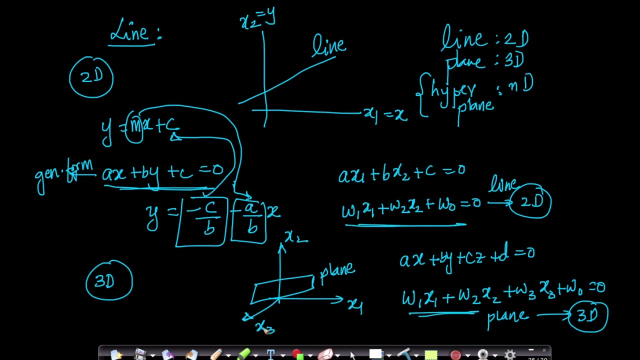 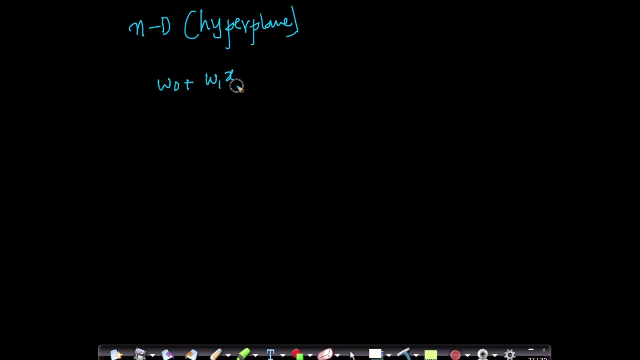 what is the equation of a hyperplane? You could have easily understood that by just looking at the form of this. This is 2D, this is 3D. Now just let us extend it and see what will it be in nd. In nd, it will be w0 plus w1x1 plus w2x2, so on, so forth. 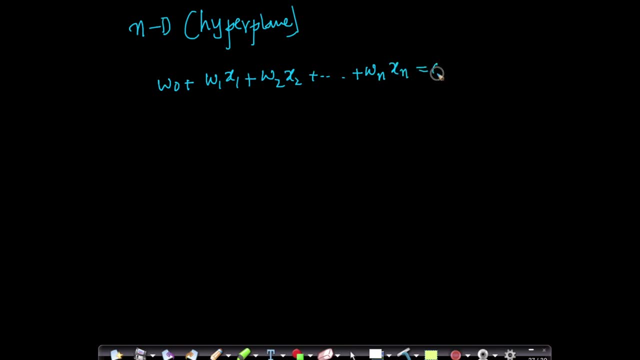 Since we have n dimensions, wnxn equals to 0.. This is the equation of an n-dimensional hyperplane. Now the immediate question we get is: this is too cumbersome to write a more concise way of doing it? Of course there is. We can use summation here. 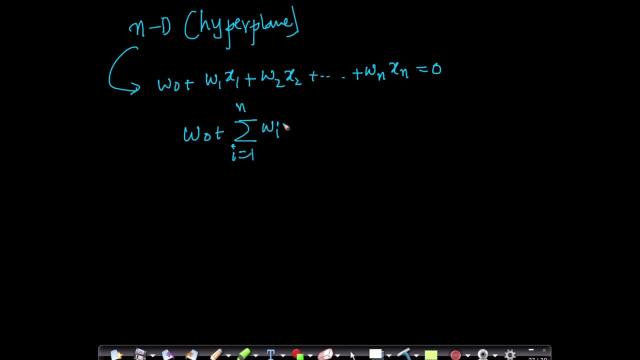 Summation: i equals to 1 to n. wi. xi equals to 0.. Now is there a better way to write this still further? This is still good. This is certainly much more concise way of writing the equation of a hyperplane in n-dimensional space than writing out this whole expression. 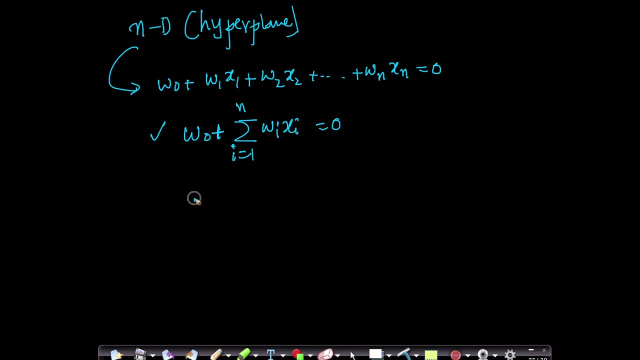 There is a slightly more interesting way of doing it, which is I can write it as w0 plus, so on, so forth. So imagine, if I create a vector right w This vector, I will call it w. So those of you who remember how to multiply two vectors or multiply matrices, you will. 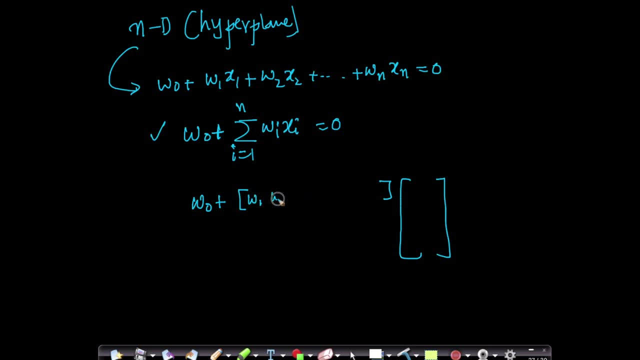 quickly recognize this. Let us assume I have w1, w2, so on, so forth. wn here. Imagine if I have x1,, x2, so on, so forth. xn here. This is nothing but a vector notation. This is nothing but a vector notation. So imagine if I have x1, x2, so on, so forth. xn here. 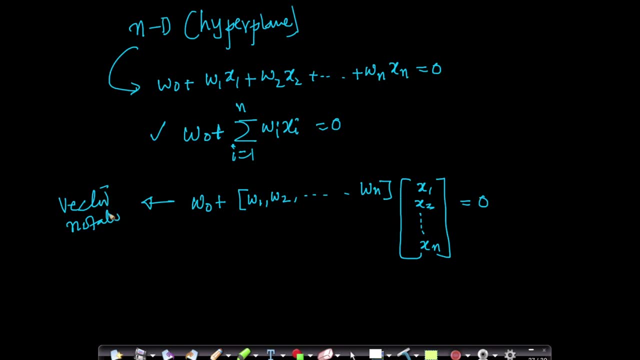 This is nothing but a vector notation. This is nothing but a summation notation. right, I am just. I am not changing any formula here, I am just changing the notation slightly. So what does this product look like? So, when you multiply this vector with this vector, 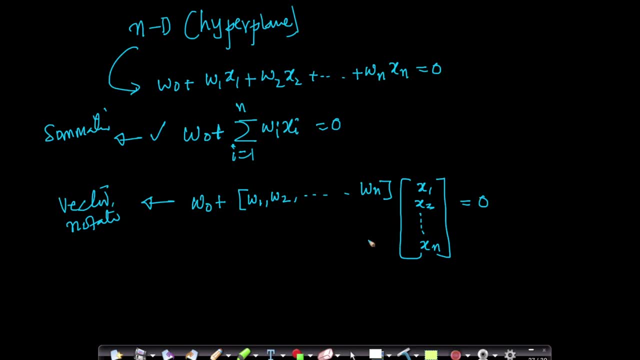 those of you who have studied basic matrices and matrix multiplication, probably in your 11th grade or 12th grade, you will easily recognize this. So this is nothing but w0 plus The first component here gets multiplied with the first component here, right, which is nothing but w1, x1. And then you add: take the second component. 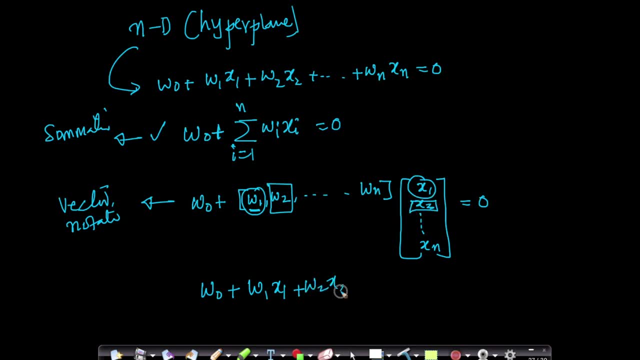 multiply it with the second component, which is w2,, x2, and so on, so forth. Take your last component. multiply it with the last component, which is wn. xn equals to 0.. So this is a vector notation of writing it And we will use this notation a lot. 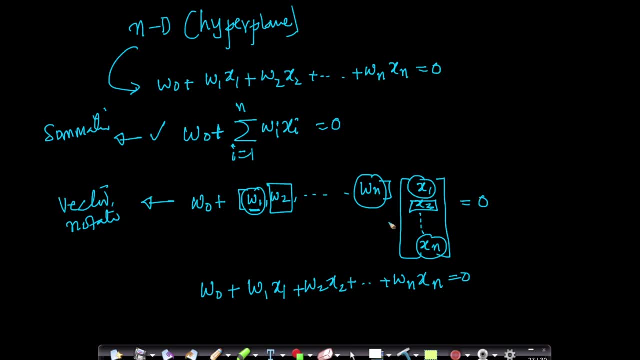 Immediately after this section, we will understand what is a dot product and we will write this in a concise form. So this is a vector notation. Now, this vector, I can, since this vector, I can think of this as a vector w. 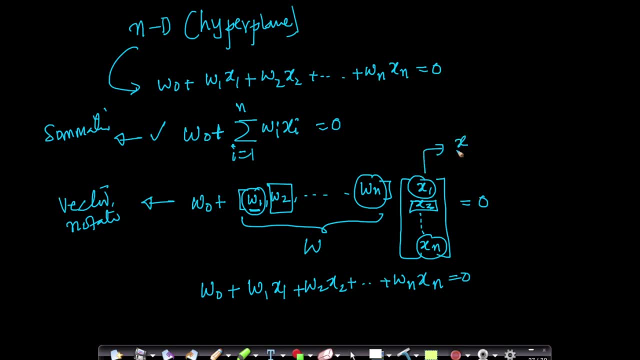 I can think of this as a vector x, right, This vector x has n rows. right, It has n rows and it has only one column. This vector w has one row and it has n columns, right. So, if you recall the vector, the matrix multiplication. 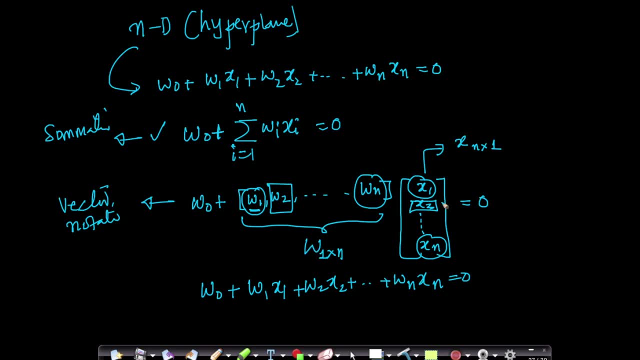 you can multiply 1 cross n with n cross 1 to get a 1 cross 1 matrix. So those of you who remember simple matrix multiplication, you will quickly understand that what we have here is nothing but a simple matrix multiplication of a row vector with a column. 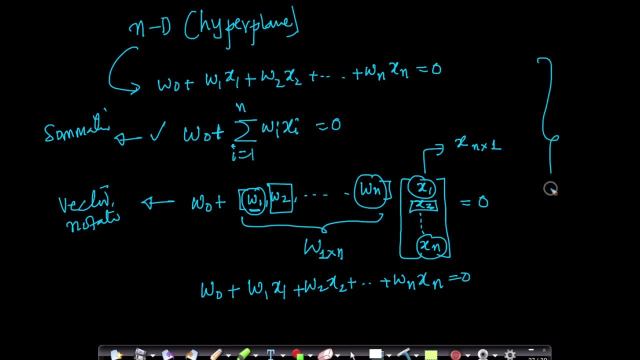 vector right. So this is how we represent a plane. We look at a plane or hyperplane in n-dimensional space. We look at many properties of lines and planes in the next few videos. Just a while ago we realized that we can multiply 1 cross n with n cross 1 to get a 1 cross 1 matrix. 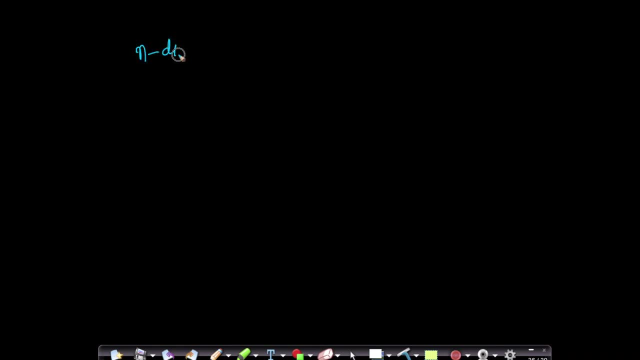 So what we can do is that the equation of a plane in any n-dimensional space is w0 plus a vector w, like this, where you have w1, w2, so on, so forth: wn multiplied by a vector like this: x1, x2.. 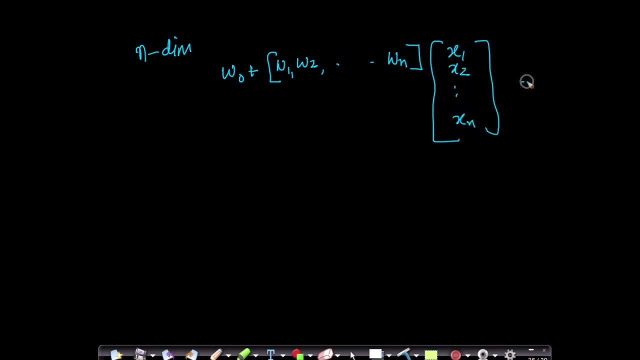 If you have n-dimensional space, xn equals to 0.. So I just told you a while ago that, given any vector, if I write a vector w, by default it is a column vector. If I say I have a vector w which is of n dimensions, by default the default convention. 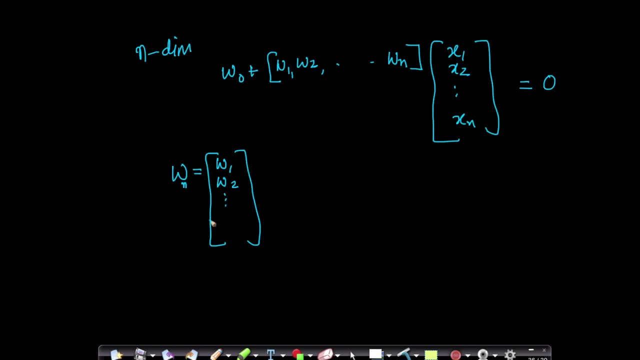 is. this is just for simplicity, to avoid confusion between whether a given vector is row vector or column vector. So the default notation is that I have n rows and 1 column. So if I write a vector x of n dimensions, I am just writing a vector here. okay, Let 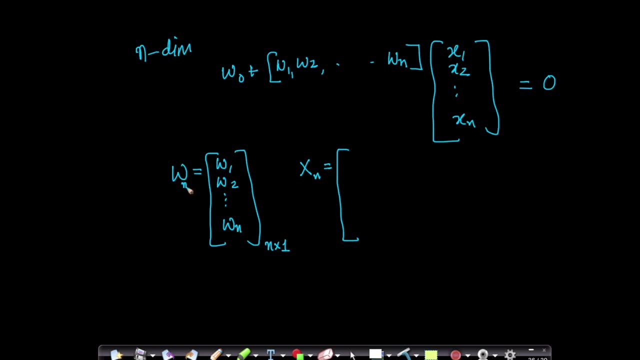 me define a bunch of vectors. I have defined a vector which is of size n cross 1.. Let us be very specific. I am also defining a vector x of size n cross 1, where I have x1,, x2,, so on, so forth: xn. 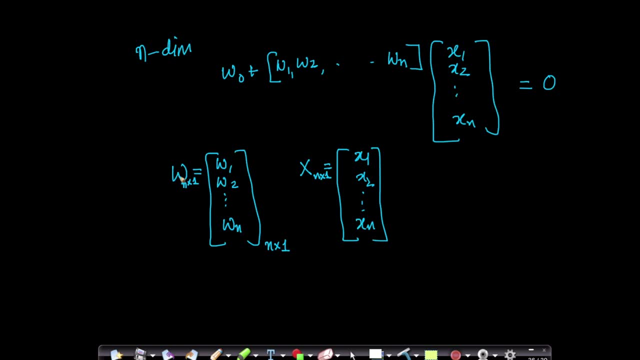 right Now, using this, using my w and x, which are n-dimensional column vectors. how can I write this equation little more concisely, right? I can write it as: w0 plus w, transpose x equals to 0.. Let us digest this. 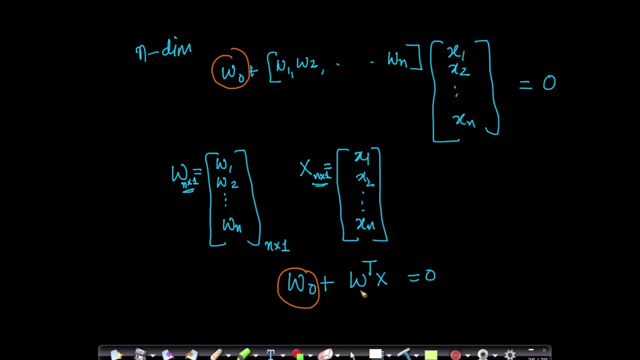 My w0,. I have just Let us copy w0 as is. Since my w is a column vector, I need to convert it into a row vector because this is a row vector, right? And how do I convert a column vector to a row vector? 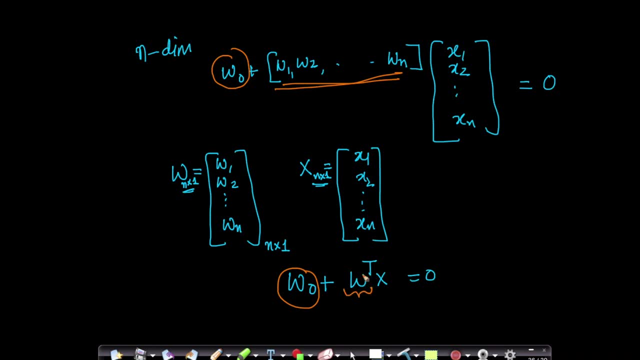 I just apply the transpose part. So your w transpose is nothing but will give you a row vector like this And your x is a column vector which is exactly like this. So what I have here in a clumsy format, I have just concisely written it as: w0 plus w transpose x equals to 0.. Of course, 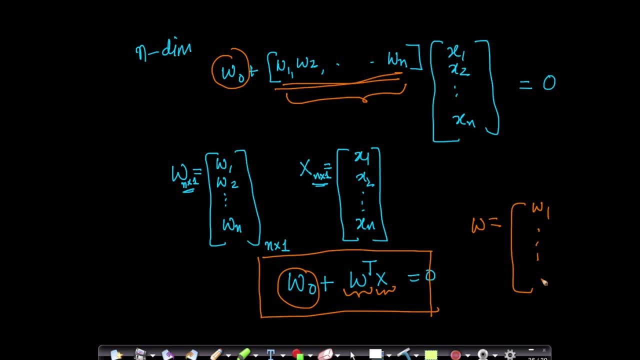 where my w is a column vector with w1,, w2, wn components And similarly my x is a column vector with x1,, x2, xn components. So if you have to write the equation of a plane again, planes are typically written with a capital pi right When you write pi pi here. 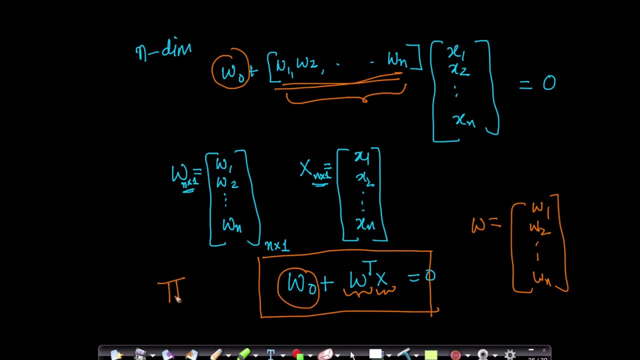 does not mean your 3.1415.. Pi. so how do you represent an unknown value In algebra? you write it with x, right? So planes are typically written as pi. okay, So a plane pi in any dimensional space can be written as w0 plus w. transpose x equals to 0.. 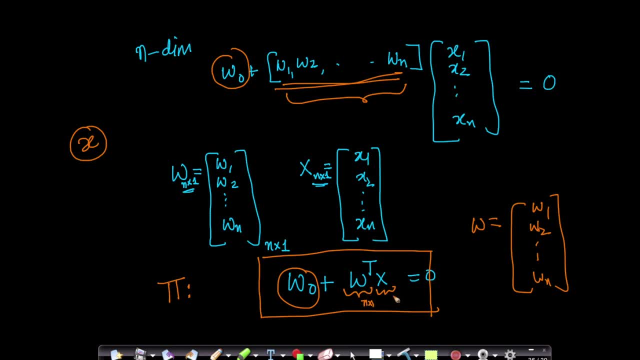 If your w is an n cross 1 matrix and if your x is an n cross 1 vector, or matrix or vector, then this is the equation of a plane in n dimensional space. right, You can write pi n to denote that this is an n dimensional plane, if you choose to. Now the immediate question I have. 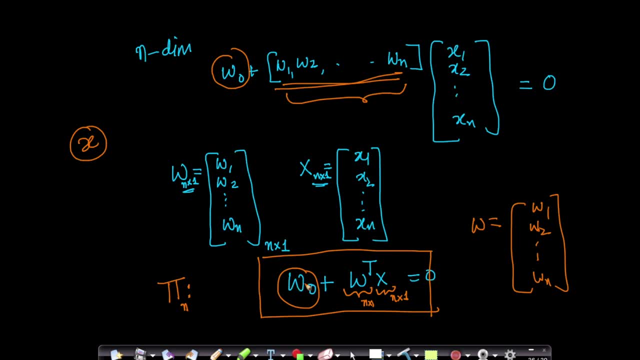 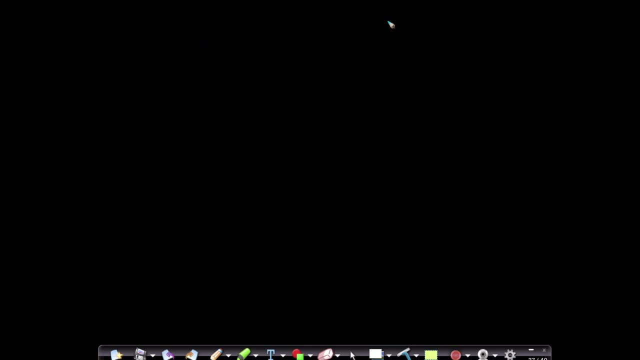 here is all. this looks beautiful, but this w0 is still hanging around here. What does it exactly mean? So let us understand what w0 actually is. So let us go to a two-dimensional geometry, because that is where we can easily understand things and we can take whatever we learn from. 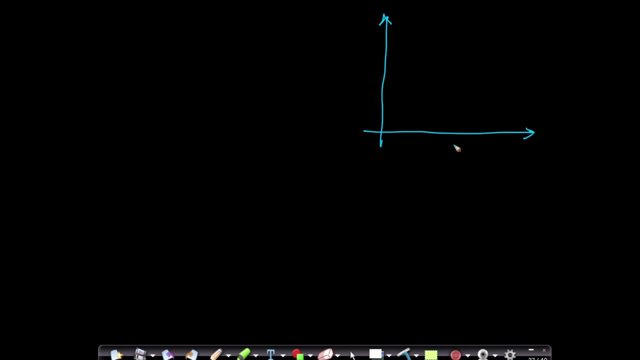 2D into a higher dimensional space. So we will always learn ideas in 2D and take it into nD using linear algebra. That is the power of linear algebra. When I first learned about it, I could not stop thinking about how beautiful and how powerful it is. Now let us say I have two axes. 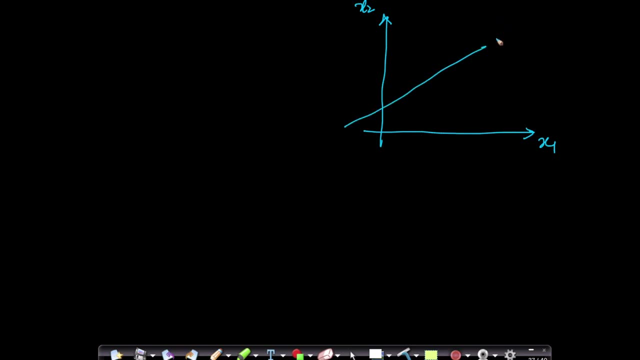 x1 and x2, and I have a line. So let us say I have a line and I have a line and I have a line like this, My equation of the line- let us assume I wrote it as y equals to mx plus c. 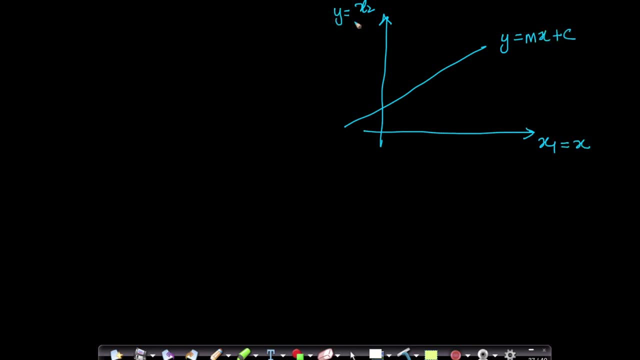 right, Where x1 is your x, your x2 is your y. Now, what is m? m is nothing but the slope of this line. m is nothing but the slope of this line, right? m is nothing but the slope of this. 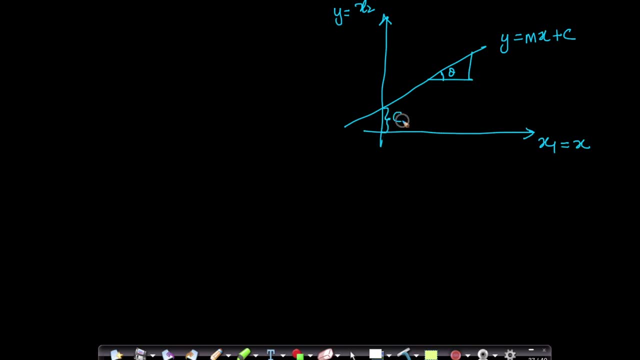 line And c is nothing, but c is called the y-intersect. c is this point On y-axis. where does my line l? where does my line l intersect the y-axis? That is called my c. It is called the y-intercept. My c is called the y-intercept, right, And my m is nothing but the. 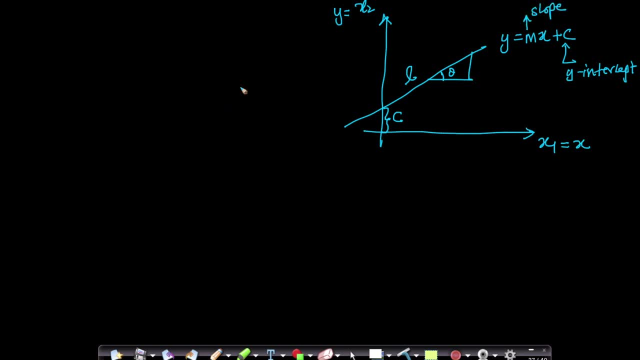 slope of my line right Now if I write the general equation of a line, let us say of a 2D line, right? So general equation of a 2D line that we saw earlier is w1, x1 plus w2, x2 plus w0. 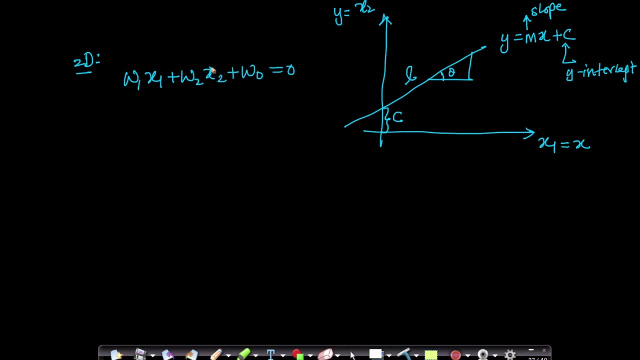 equals to 0.. Now let me just rearrange the terms here and I can write it as: x2 equals to minus w0 by w2, minus w1 by w2, x1, right Now, what is happening here? This is nothing but. 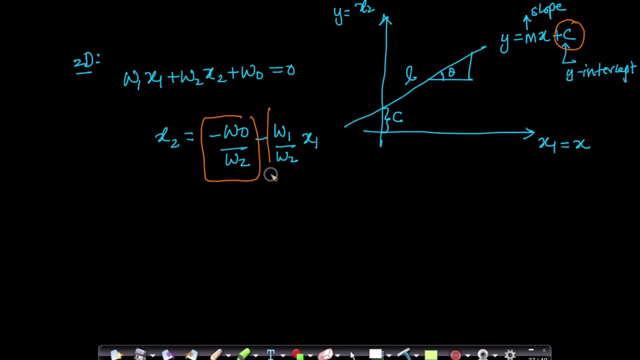 my c right. This is nothing but my c, This is nothing but my y right And this part is nothing but my m and my x1 is nothing but x. right Now, if a plane is passed, if a line is passing, 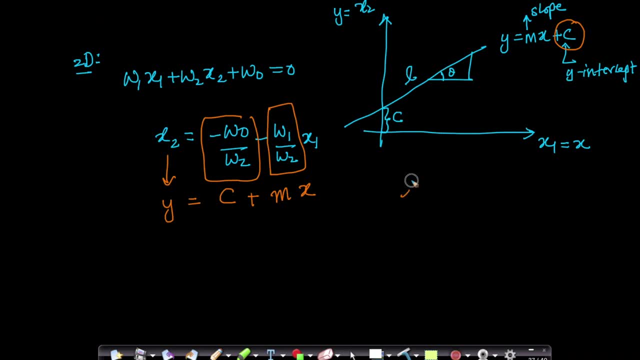 through origin. okay, So if this line l, if line is passing through origin, if it is passing through origin, what happens to c? c becomes 0, right, Because this line would have. so imagine we had a line which was passing through origin. What is its y-intercept? 0, right, Let us assume. 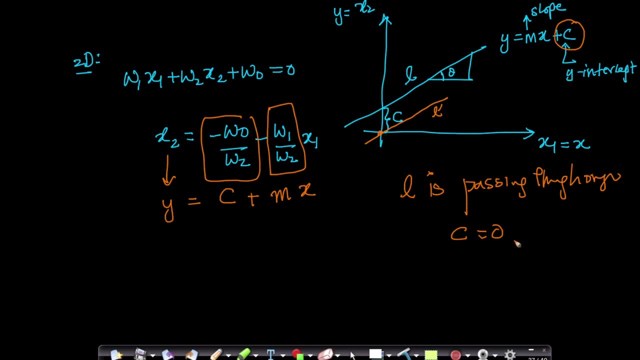 I have a line l dash. If it is passing through origin, the c is 0. And if c has to be 0, your w0 has to be 0, because c is nothing but minus w0, by w2.. And if c is 0,, if c equals to 0, that implies in my general form, in my general notation: 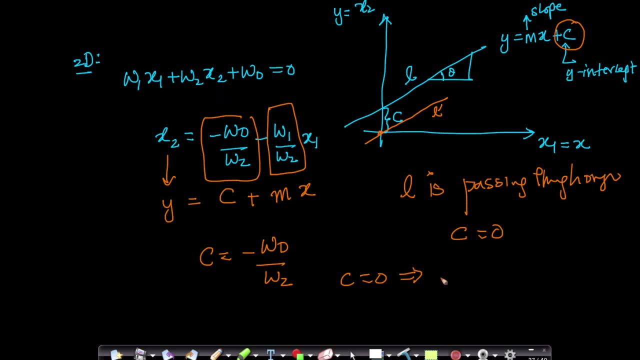 here in my general notation, or the general equation of a line that implies that my w0 equals to 0. So what we learn from this is: this is a general equation of a line, But if I have to write the equation of a line that is passing through origin, okay. Suppose if I have to write: 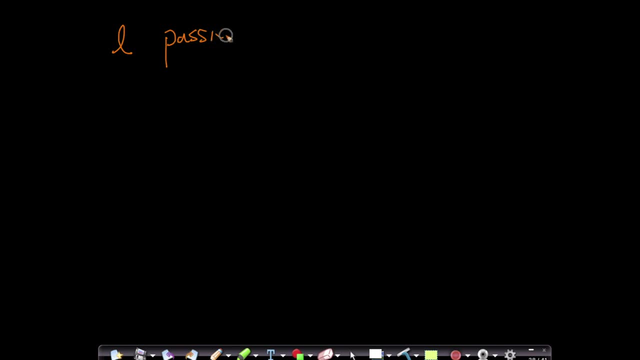 suppose I have a line, l passing through origin. Passing through origin, intuding. okay, What will its equation be? By just making my w0 equal to 0, what will my equation remain? My equation will remain: w1, x1 plus w2- x2 equals. 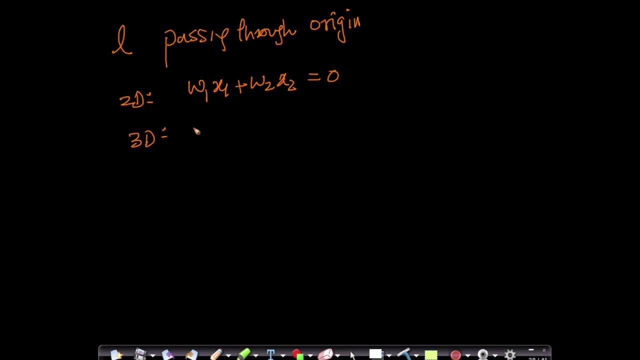 to 0.. What about 3D? Same terminology. My w0 basically becomes w2, x2 plus w3, x3 equals to 0.. In 3D it becomes a plane, of course. Right, This is a line, And in higher dimensions it becomes a hyperplane, right In the n-dimensional. 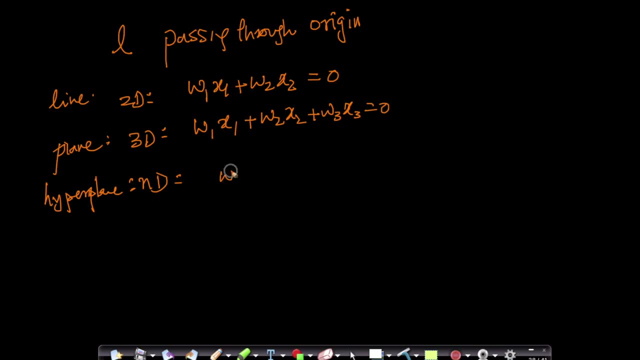 space. what does this become? This becomes nothing but w1, x1 plus w2, x2, so on, so forth. wn, xn equals to 0, which is nothing but w transpose x equals to 0.. This is a very, very concise way of writing the equation of a line. 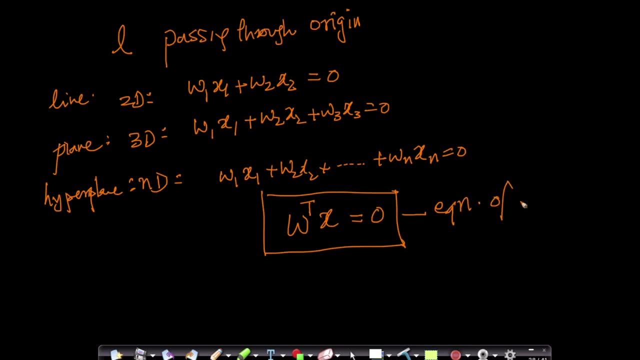 Of a plane. sorry, This is an equation of a plane. Of course this plane is passing through origin. This is an equation of a plane passing through origin. If it is not passing through origin, then the equation of the plane will be w. transpose x plus w0 equals to 0, okay. 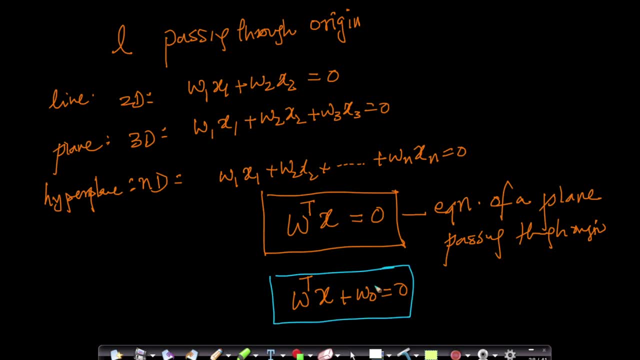 So this is the equation of a line not passing through origin. If it is passing through origin, it is nothing but w transpose x equals to 0. Such an elegant term, See using the concept of a transpose, using the concept of matrix of vector multiplication. 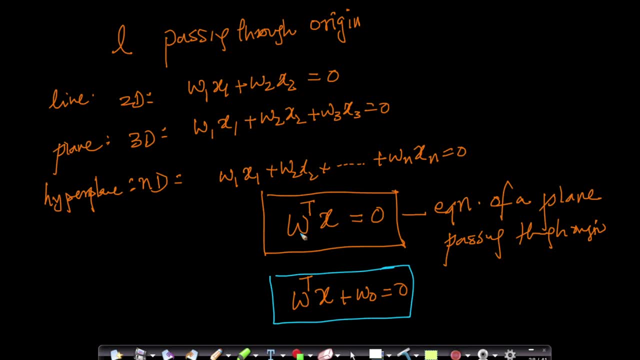 we wrote the equation of any dimensional hyperplane in a very, very concise, very, very elegant form. Of course, you have to add the w0 term if it is not passing through origin. Now let us understand the equation of a plane in a new way, using a slightly different geometric. 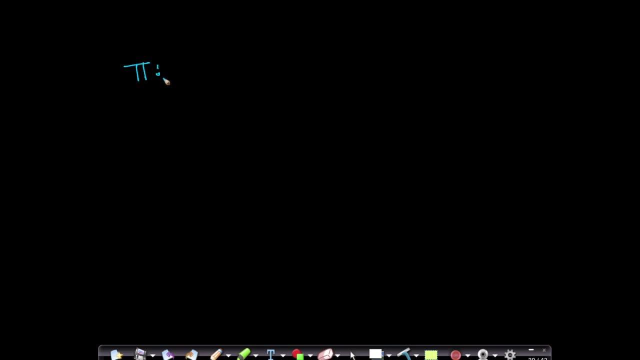 interpretation. So let us assume I have a plane pi. It is an n-dimensional plane And this plane passes through origin, which means its equation will be: w transpose x equals to 0, where w is nothing but a column vector with w1, w2, so on and so forth, wn. 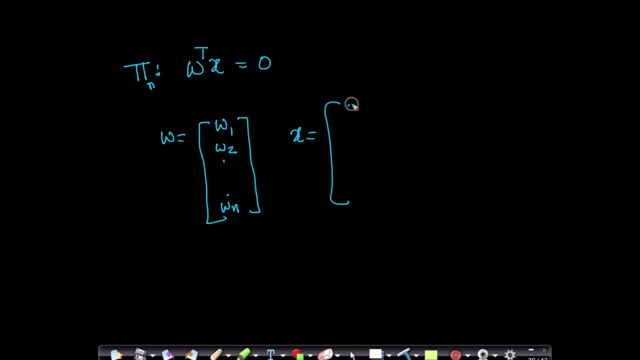 And x is also a column vector corresponding to your n dimensions. right Now, if this is the equation of plane, let us try to interpret it slightly differently. Forget about the fact that this is the equation of a plane, right? So let us see if this is the equation of a plane. 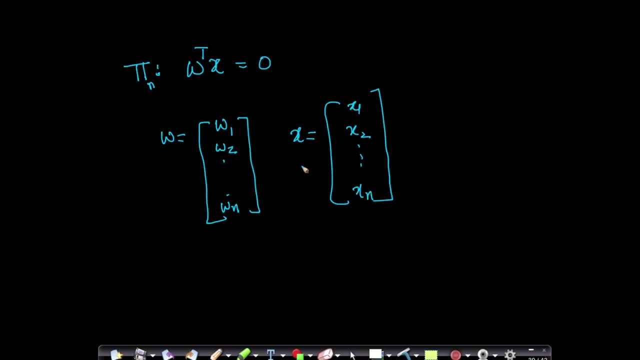 and if this is the equation of a plane, we will try to interpret it slightly differently to the plane. just for a second, Let us assume w and x are two vectors. right? We know that w dot x is nothing but w transpose x, and we know that w dot x is also can also be written as the length. 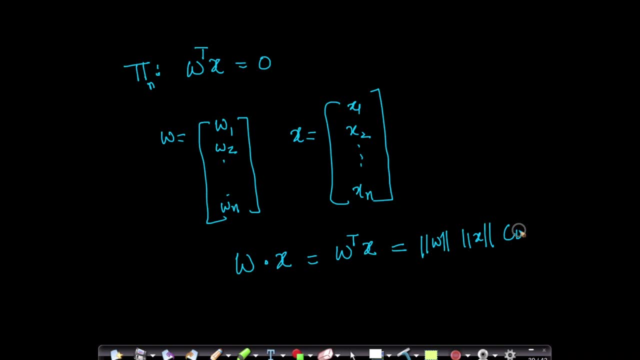 of w, the length of x and cos theta, where theta is the angle between w and x, right? So here, instead of looking at w and x as part of an equation, I am just looking at w and x as two vectors, right? This is the beauty of linear algebra. So w is just I can think of. 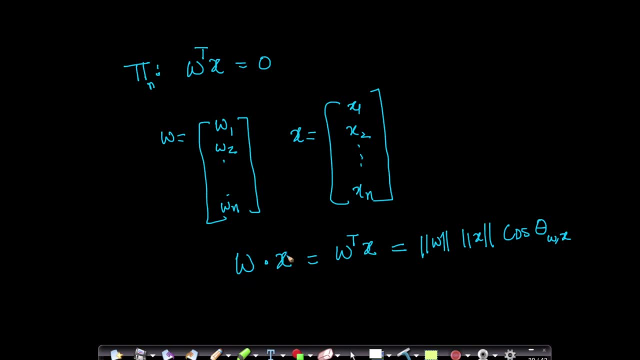 it as an n-dimensional point, so is x an n-dimensional point? So if these are two points, if w and x are two points in an n-dimensional space, let us assume this is w and let us assume this is x. this is the angle between them, theta right. We said that this. 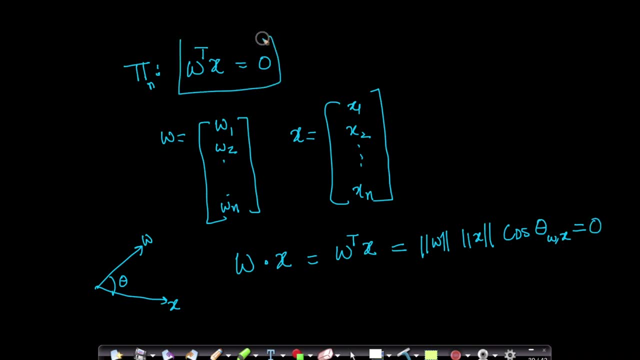 is equal to 0 for a plane. right? This is the equation of a plane: w. transpose x equals to 0. So the moment this is equal to 0, you know that your theta, the angle between your w and x, becomes 90 degrees, right? We discussed this, right? If w? 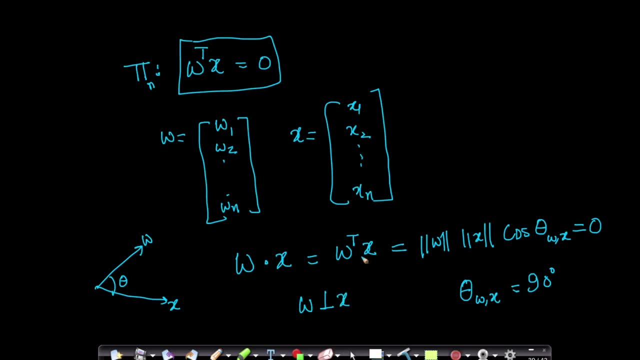 is perpendicular to x, then w transpose x equals to 0 and that implies that your theta between w and x equals to 90 degrees. right, With this, let us connect. let us understand a different way of interpreting this equation. Suppose I have a plane. okay, I will write this plane as pi. 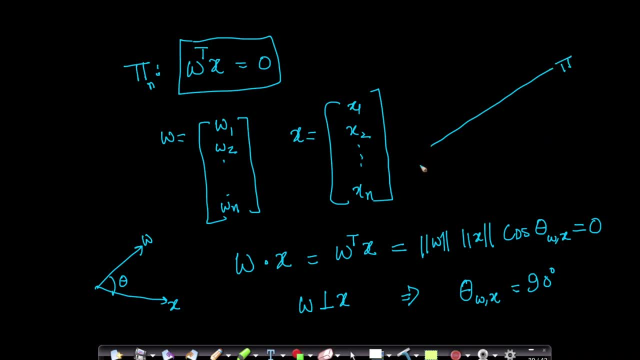 Of course, I do not want to draw a three-dimensional plane, So, since a line or a hyperplane, everything is a linear surface, just for simplicity, I will draw it like this instead of drawing a plane, because this is easy to interpret and easy to understand, because it is a. 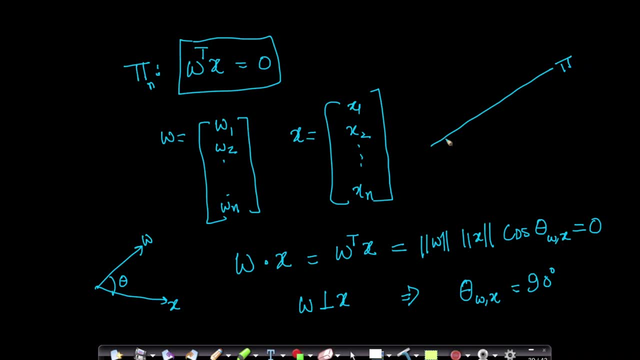 two-dimensional surface on which I am drawing things, drawing a line is much easier. Let us assume this is origin. We said this plane is passing through origin. right, Let us assume this is origin. okay, Let us assume this is any point x1 on this plane. right Now we know that. 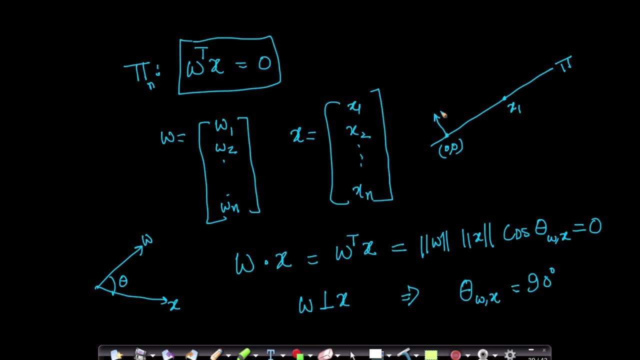 w is perpendicular, So let us assume w is like this. Let us assume w is a vector like this which is perpendicular to plane. I will connect all the dots. Please bear with me Now. if w is a vector which is perpendicular to your plane and at origin, let us assume w is a vector which is perpendicular. 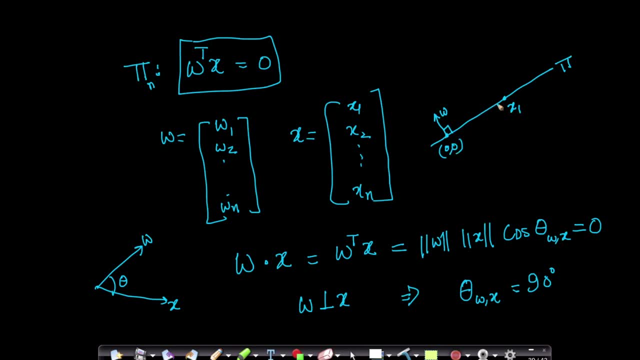 to your plane pi passing through origin. just for simplicity, Now let us assume x1 is a vector. x1 is a point. right, A point can be thought of as a vector right Now, since these two vectors, w and x1, are perpendicular. w dot x1 equals to 0,. 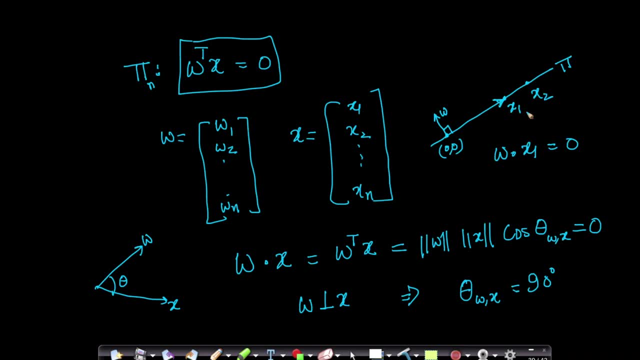 so for any point on this plane, if we take any point on this plane, if w is perpendicular to this plane, then w dot x1 equals to 0 and that is what we are calling the equation: the plane Instead of this x. if I replace any point on the plane instead of this x here, if I replace with any. 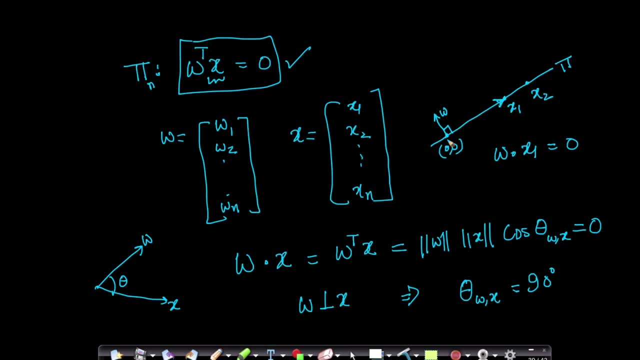 point on the plane, then my transpose x equals to 0, because my, if, my, w. so if, if w is perpendicular to my plane, then w transpose x, i. so then then w dot x i equals to 0 for all x i which belong to my plane. 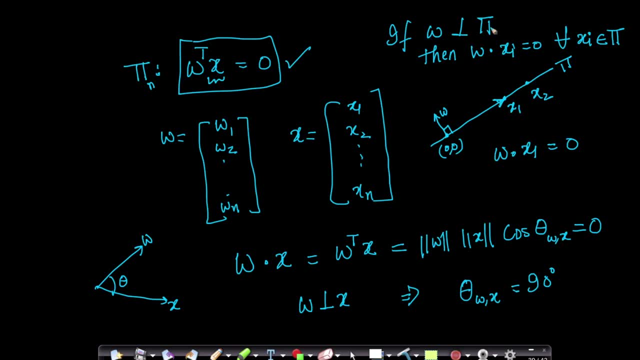 let me read it in english again: if w is perpendicular to my plane pi, then w dot x, i will be 0 for all x i belonging to the plane right. this how it is always important to read equations in english. that simplifies things for us. now, having said that, one way to interpret. 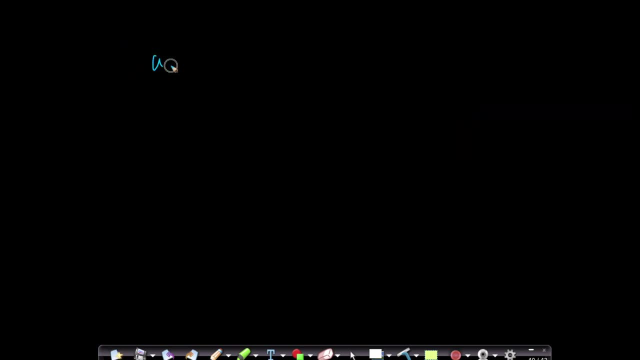 interpret this equation. one way to interpret your w- transpose x equals to 0- equation is that you have a plane, pi, which is passing through origin, and w is nothing but a vector which is perpendicular to your plane. okay, this is one way of interpreting what w is. 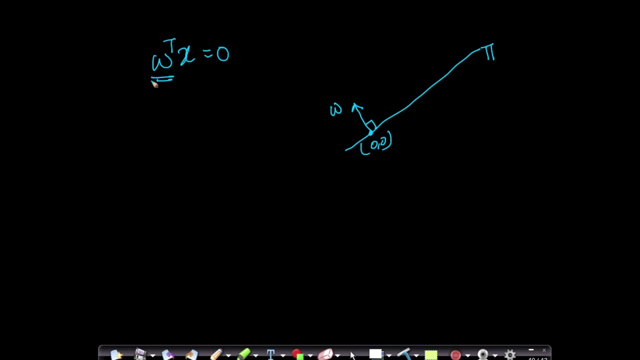 this is a very simple and elegant interpretation of w, because till now we did not explain what w is geometrically. we just, we just derived this w from your a, x plus b, y plus c equals to 0 type of equation in 2d, but we never said what does w actually mean geometrically? so 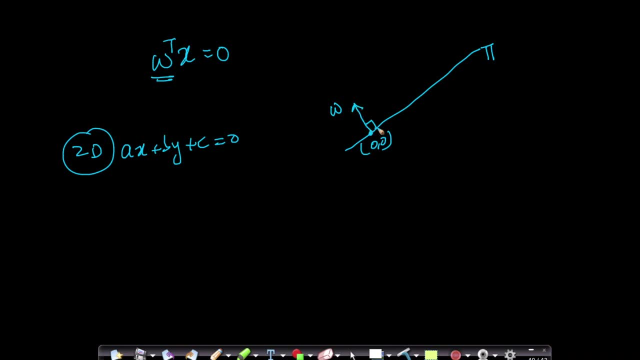 what w means geometrically is nothing, but it is a vector which is perpendicular to this plane at at origin. that is important, okay. so one thing that people often represent w is so because w or the unit vector w. what is the unit vector w? unit vector w is nothing but w by the length. 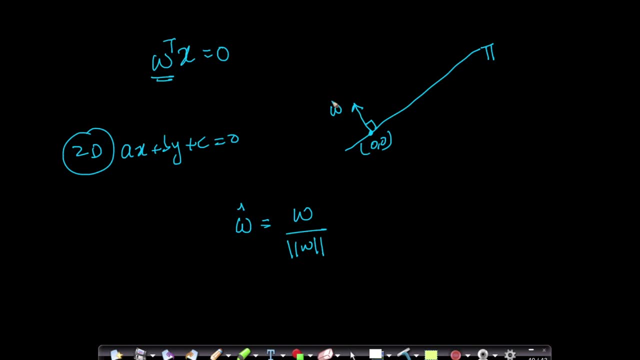 of w right. so because instead of w, let us assume i have unit vector w, even then my w dot any x i will be 0 for all x i belonging to my plane right. oftentimes a plane pi is represented with a vector, with a unit vector w cap. oftentimes it is just written as w okay.